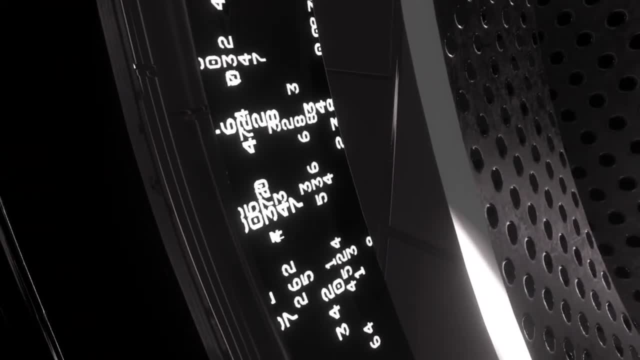 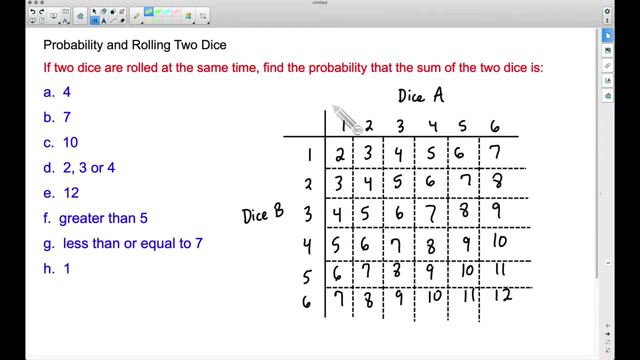 All right, in this video we're going to find the probability of rolling two dice, But in this example, if two dice are rolled at the same time, we want to find the probability that the sum of the two dice is one of these things in here. So before we dive into the examples, here is a common. 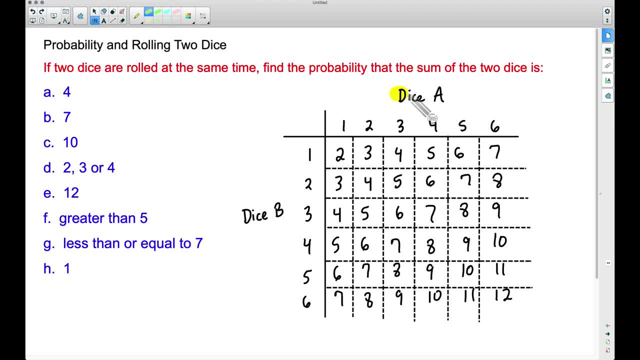 chart And you can Google this chart as well. But we have dice A, This is our first dice, First die, first dice, plural, singular, whatever. But when we roll a dice we can land on a one, two, three. 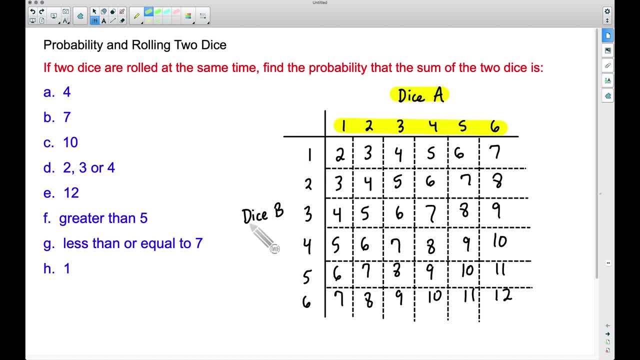 four, five or six. So that's our first die. Dice B: we can land on a one, two, three, four, five or six. Now what we're curious about is the sum When we roll these two dice, add the two numbers. 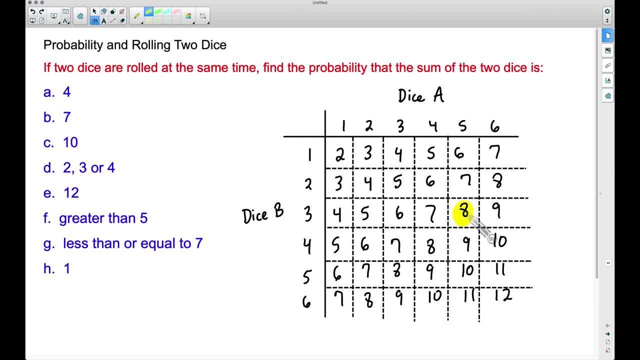 together. what do we get? For example, let's look at this eight. How do we get this Eight here? This is a sum And to get this eight that means we rolled a five on dice A and a three on dice B. But there's other ways of getting an eight. For example, look at this one down here: 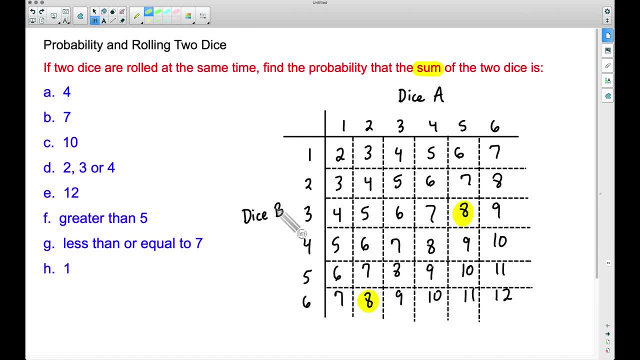 This eight here comes from rolling a two on dice A and a six on dice B. That's how we get that eight. Notice this one up here. we rolled a six on dice A and then we rolled a two on dice B, So you know. 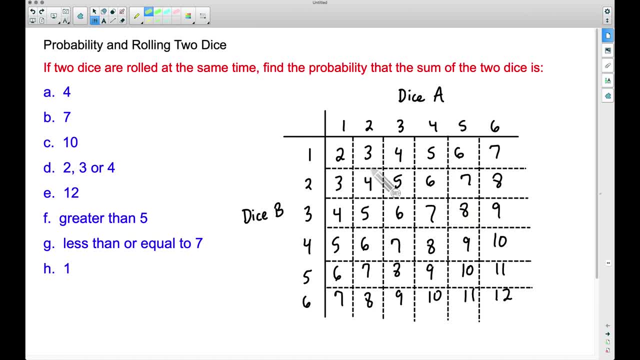 you're trying to look at this as like a little Excel sheet or a spreadsheet. You know we got all of these right here. What do they have in common? That means we've rolled a one on dice B, but we rolled a. 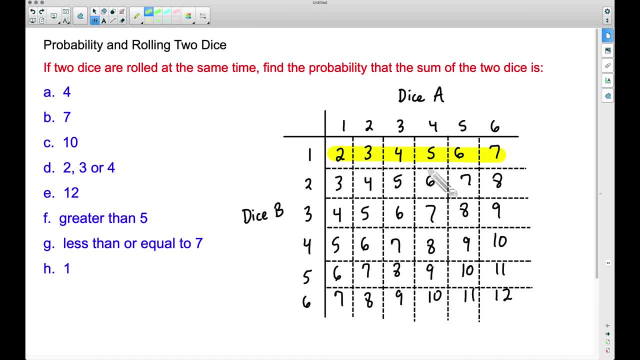 different number on dice A and that's how we're getting these different sums here. Now, if you look inside of all of this stuff right here, there are 36 possible sums, 36 total outcomes here, And the first question says: find the probability. find the probability that the sum of the two dice 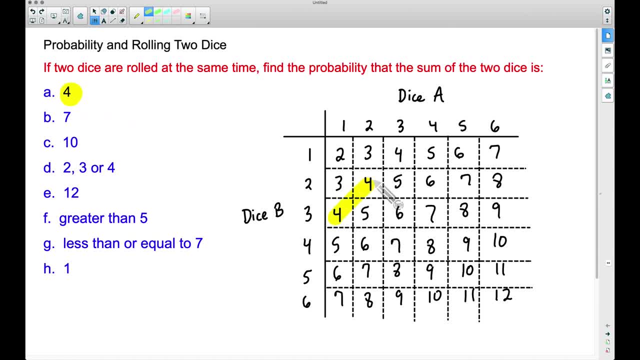 is four. Well, if we look at the fours, these right here, and no, no, no and no, don't talk about that one and that one. No, we don't talk about those. That's just the actual numbers that we get on the dice. 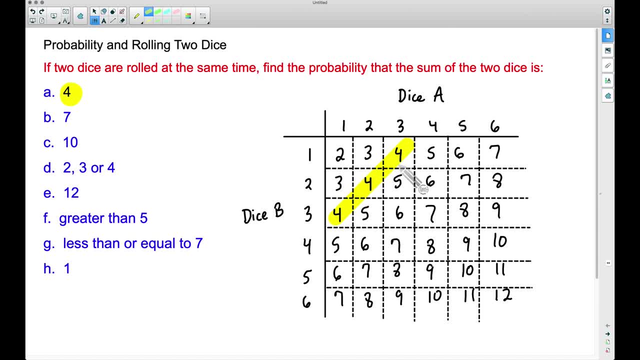 But these are three possible ways to get a sum of four. We can roll a three on dice A, a one on dice B. that will give us a four. We could roll twos on both of our dice to get a sum of four. or we could roll a one on dice A and a three on dice B to get that sum of four. 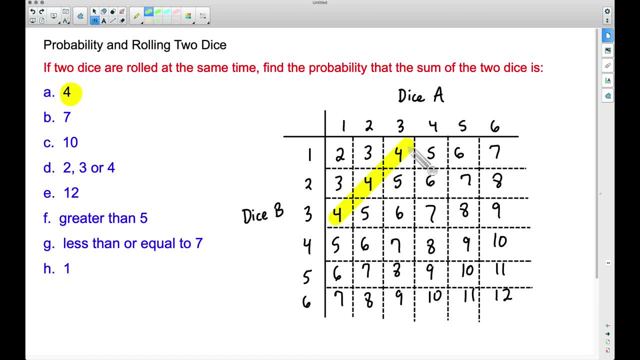 So that probability is going to be three possible ways out of a total of 36.. So that probability is going to be three out of 36.. And if we reduce that fraction, divide the top and bottom by three, we get 112.. So that's the probability of rolling a sum of four when you roll two dice. 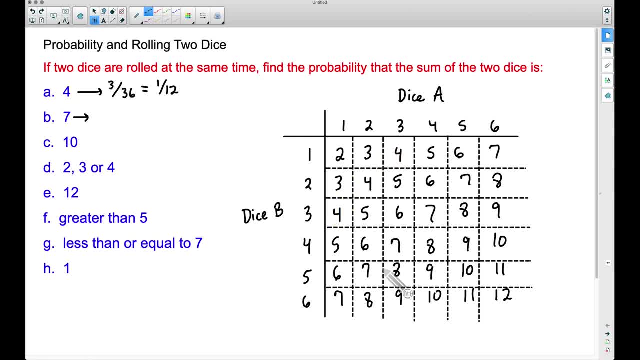 All right. what about the probability of rolling a seven? Well, we got a bunch of sevens. As a matter of fact, that is the most probable sum that you're going to get when you roll two dice. there's a whole bunch of ways to get a seven. we can roll a six on dice b and a one on dice a to get that. 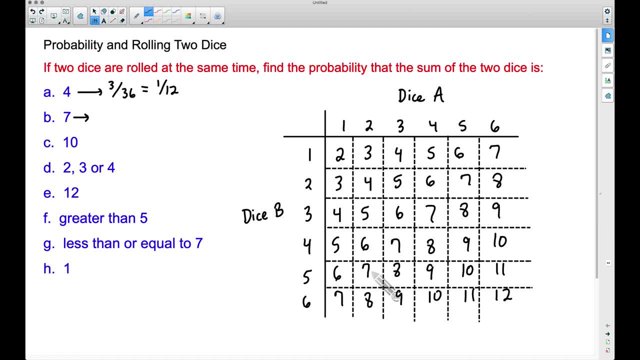 seven there, and you know, then we have fives and twos, twos and fives, threes and fours, fours and threes, and you know this other six on dice a and one on dice b. there are actually one, two, three, four, five, six possible ways, six out of thirty six. dividing the top and bottom by six, we reduce this. 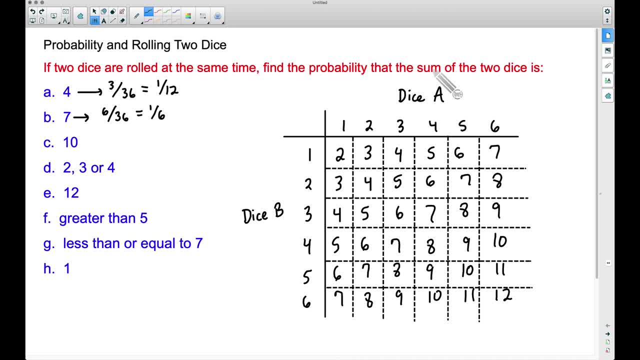 fraction to one six. therefore, the probability of you rolling a sum of seven on two dice is one six. what's the probability of rolling a sum of ten? well, down here we got one, two, three possible ways, and again that's the same thing as what we had up here: three out of thirty six. that reduces to 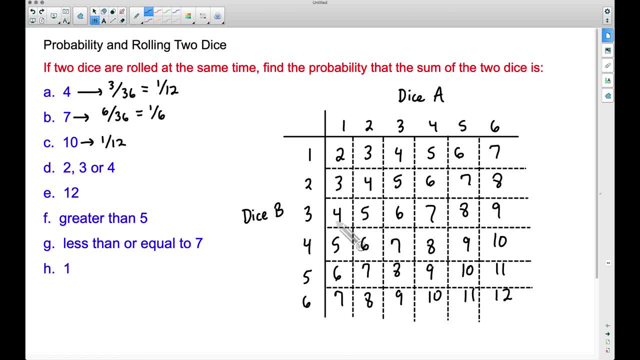 one twelfth. with that said, the probability of you rolling a sum of four is the exact same thing as you rolling a sum of ten. when you roll two dice, all right, this next one. here we have our or statement: what's the probability of rolling a sum of two, or three or four? we're talking about this little section right here. 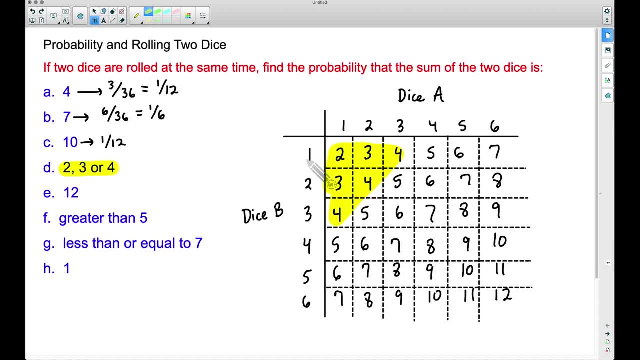 rolling a sum of two. there's only one way to do that. you roll snake eyes. that's, uh, rolling a one on both dice, but we're talking about a two or three or four. that's a total of six ways if you add up all those, and we've already seen that probability up here. 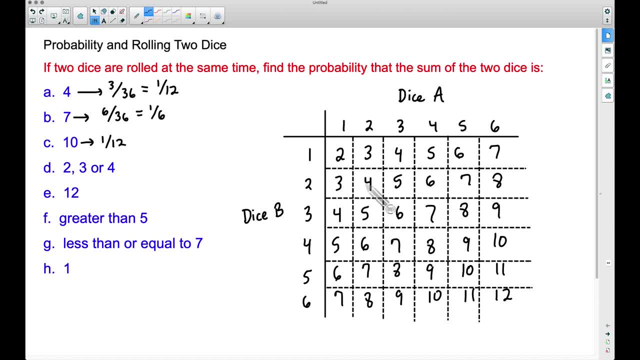 with the seven, six ways to get a seven. where there's six ways here to get a sum of a two or three or four, and we said that simplifies to 1: 6. what's the probability of getting a sum of 12? there's only one way you can do that. you. 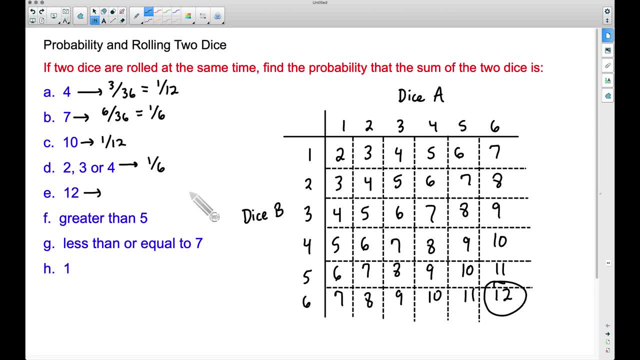 have to roll a 6 on both dice a and dice B. that probability is 1 out of 36, very unlikely. moving along, what's the probability of rolling a sum that is greater than 5? now, it has to be greater than 5. it can't be equal to 5 or less it. 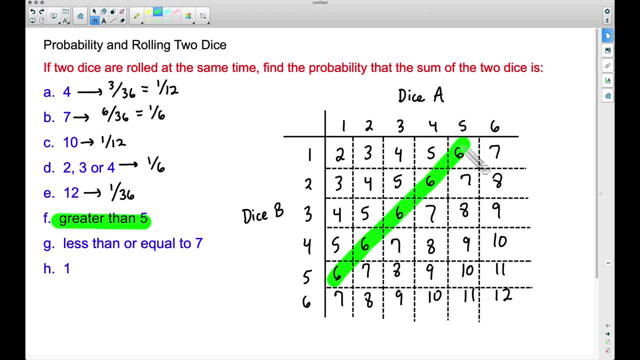 has to be strictly greater. so we're talking about these sixes right here, these sevens as well, the eights, nines, tens 11s and this 12. so let's just add up all these count how many things that I have shaded in green. so one, two, three. 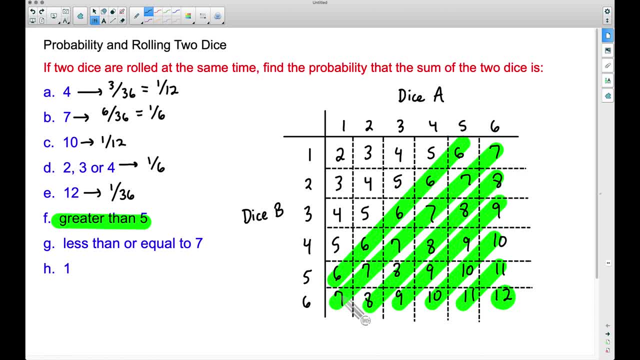 four, five and then there's six right there. that makes 11 plus 5 more makes 16, 17, 18, 19, 20, 21, 22, 23, 24, 25, 26. that is going to be 26 out of 36. pretty doggone likely that. 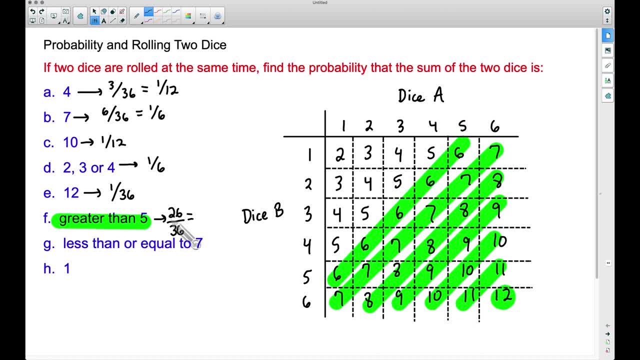 you're going to get a sum greater than 5 when you roll two dice. if we divide these by 2, we get 13 out of 18. now, another way that you could look at this: 26 out of 36. if we look at the ones that we've got here, we've got the ones that 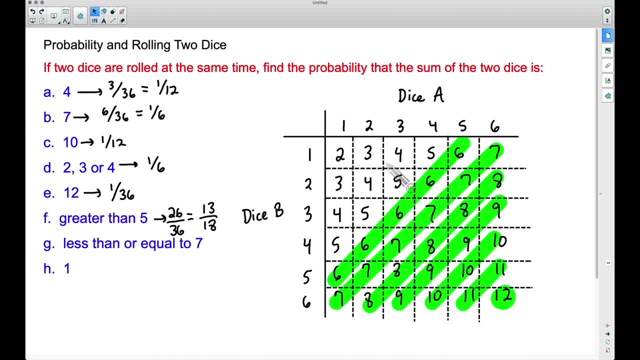 we did not highlight 1, 2, 3, 4, 5, 6, 7, 8, 9, 10, 10. there are 10 ways that we will not get a sum that's greater than 5, so that leaves you with the remaining 26 think. 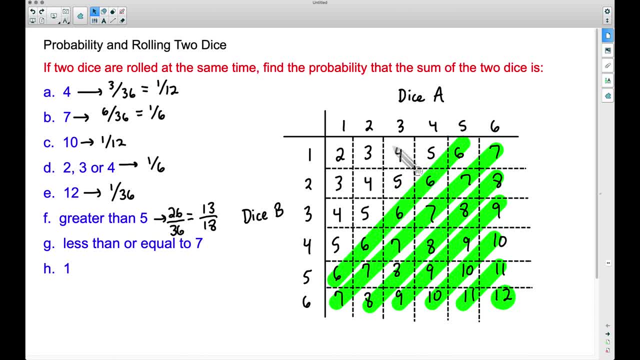 about that. there's 36 ways in all. if there's 10 ways, we cannot do it. that leaves us with 26 ways that we can do it, so just two more left here. what's the probability of getting a sum that is less than or equal to 7, less than or? 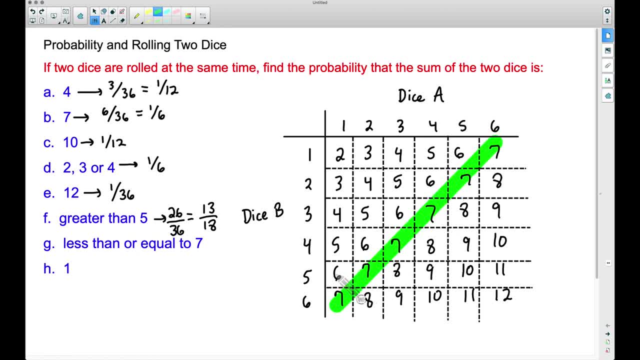 equal to seven means we can be equal to seven here and we can be seven or less, So all of these that we see right along here. So either you can add up the greens or you can add up these pieces. we did not shade and subtract that from 36.. I'm going to do that in this case. So we got one, two.